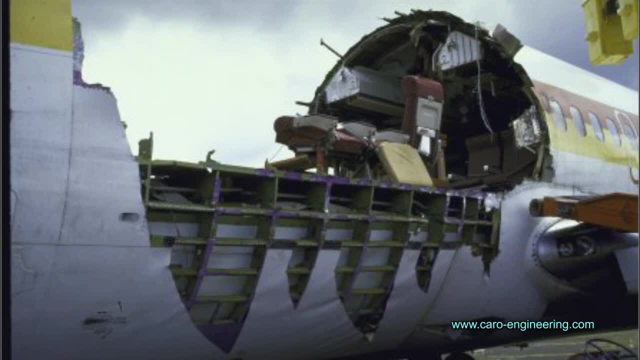 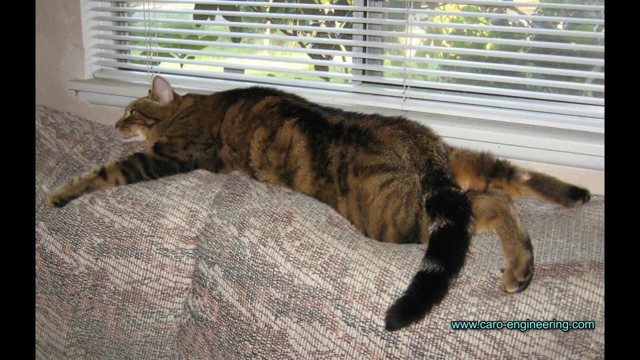 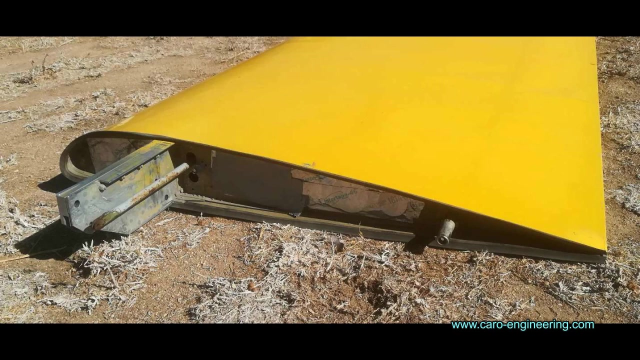 First of all, what does fatigue mean for structures? Everyone is personally familiar with fatigue. After strenuous exercise, you feel worn out or sleepy. It is similar for structures: When they are worn out after a lot of flying activity, they would like to be retired from service. If that does not happen, they eventually break. 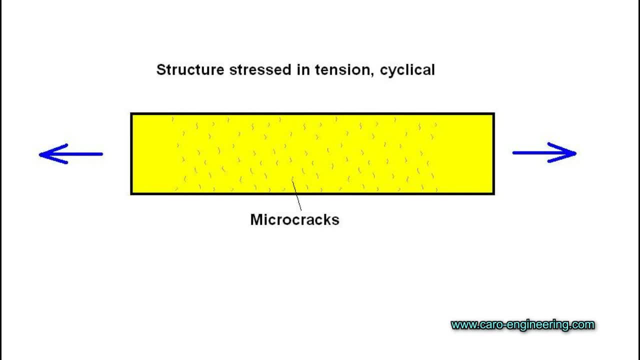 To explain why this happens, I will use this piece of aluminum as an example. It is repeatedly stretched and released for many thousands of cycles. During each cycle, where some of the stress is in tension, a very small amount of damage is caused. 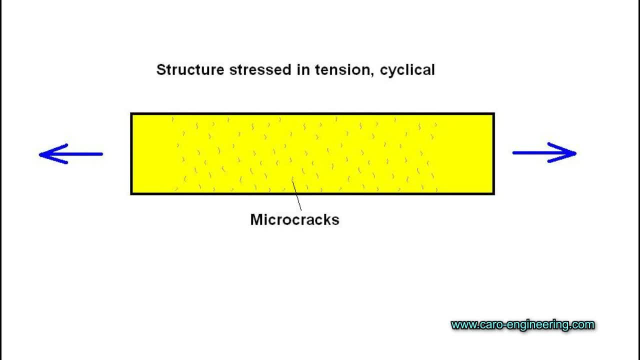 Sort of like tiny cracks. By the way, only tension causes problems. Loads that produce only compression stress do not cause fatigue damage For a long time. these cracks are so small that they are not visible. If the part was loaded to failure after about 10,000 of these cycles, it would fail at a somewhat lower ultimate stress than a part that had never been in service. 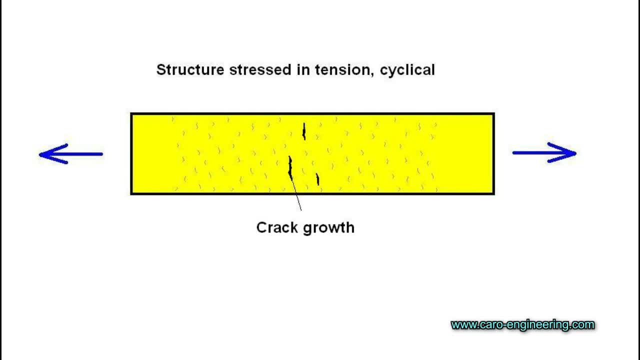 If the stretching cycles of the part are continued, the damage is reduced. If the stretching cycles are continued, the damage is reduced. If the stretching cycles of the part are continued, the damage is reduced. The damage continues to accumulate and the micro-cracks turn into real cracks that eventually may become visible. 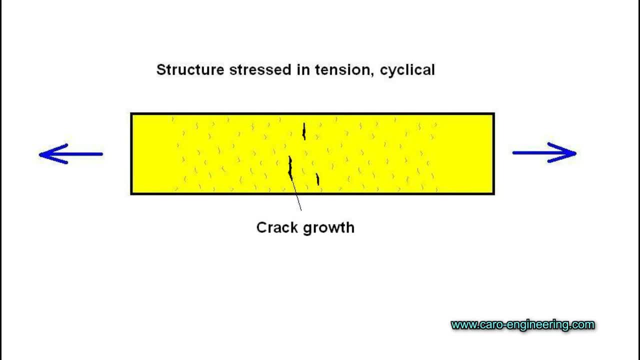 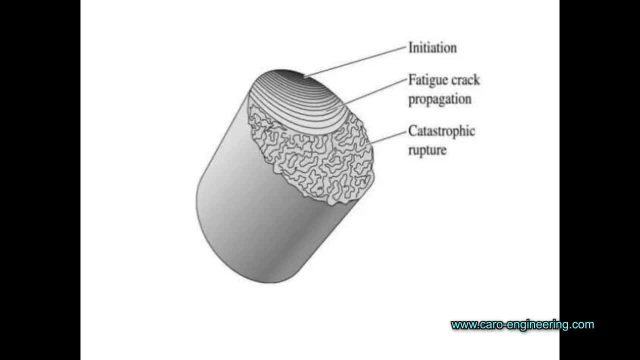 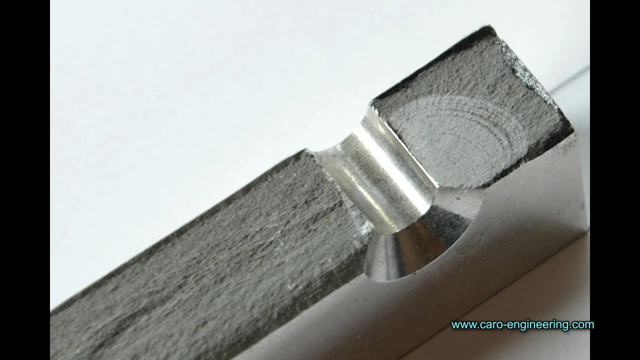 The cracks may be tiny on the surface but can progress unseen internally. Once the damage is done, it cannot be reversed or removed Eventually. when a crack reaches a critical size, it propagates suddenly and the structure fractures. The number of cycles after which a part fails on the normal level is reduced. 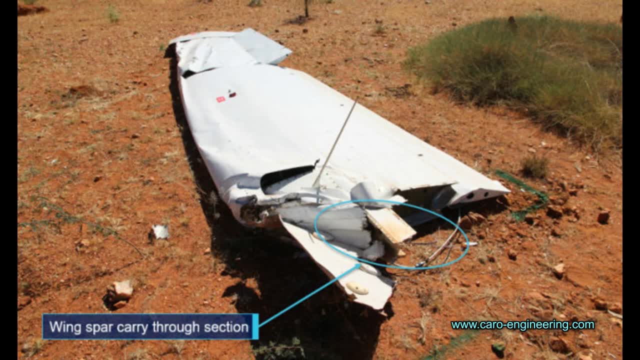 The 33% level of the damage becomes a ridiculous height. The inner frame will involve work of swaggingョing, work of. I want to mention the most important ones here: pourrait, which has the largest influence If the loads are high and the part is stretched close to its yield strength on every cycle. 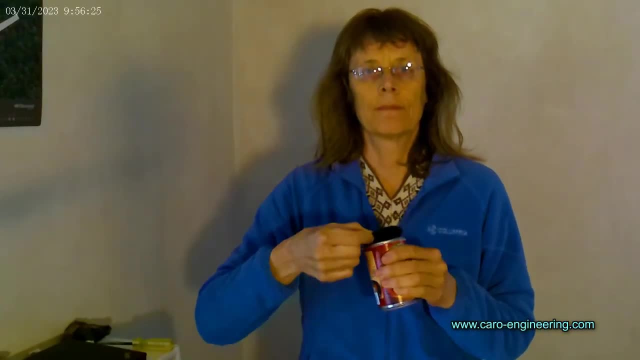 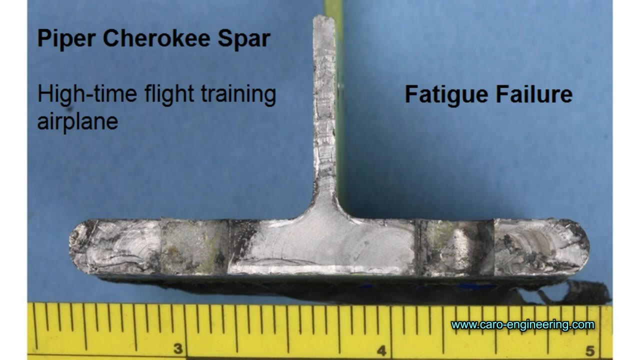 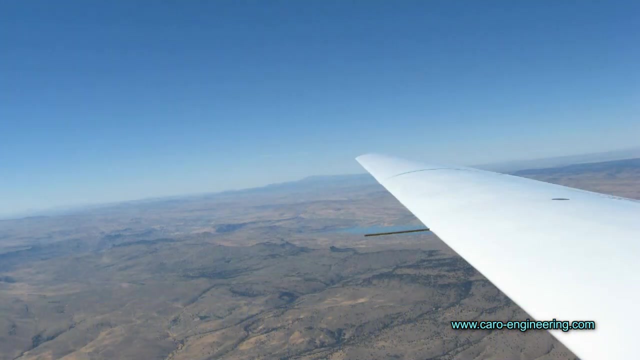 it will fail after very few cycles, as I am here demonstrating with this lid of a metal can. There is very little or no warning at all before fatigue failure. therefore the consequences are often catastrophic. If the stress level is low, the part can endure hundreds of thousands of cycles Below a certain 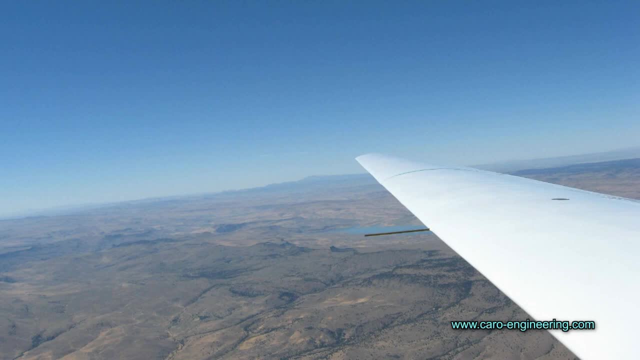 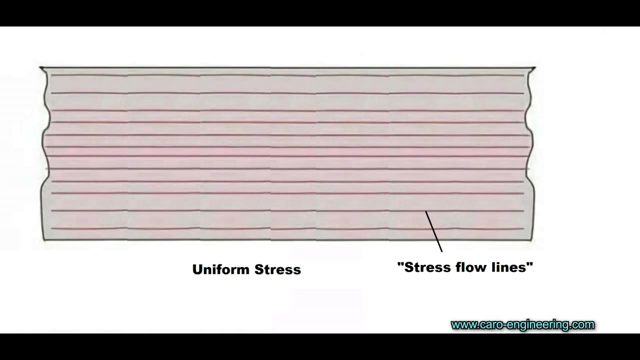 stress level. some materials can even have an unlimited fatigue life. The design of the part also has a major influence on its fatigue life. A bar with a constant cross-section has a uniform stress distribution and is the ideal case for a long fatigue life. If it had a hole or a notch, there would be stress. 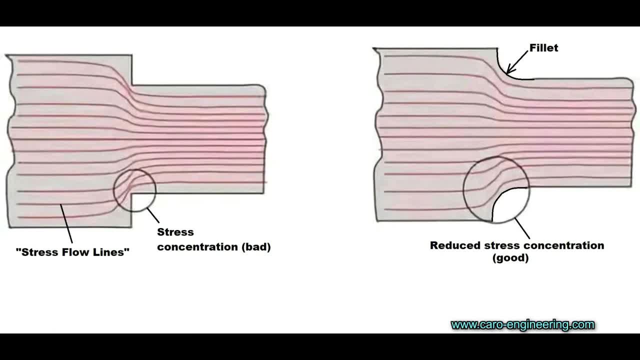 concentrations. The fatigue damage at a stress concentration can be many times higher than in a part without this. If you take a metal rod and cut a notch into it with a saw and then bend it, the stress concentration can be much higher than in a part without this. If you take a metal rod and cut a notch into it with a saw and then bend. 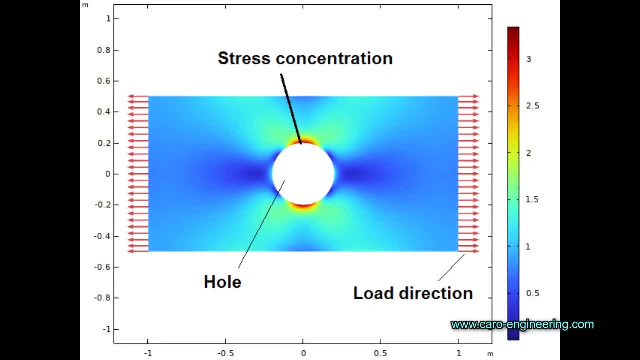 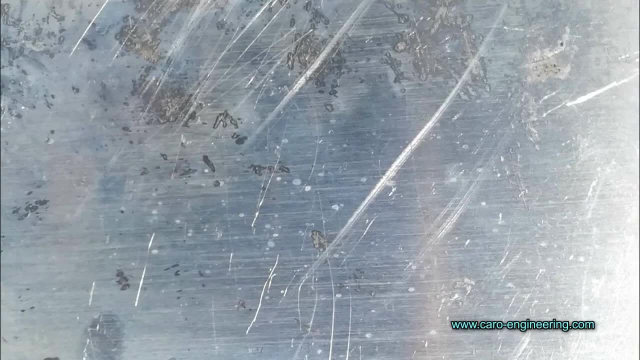 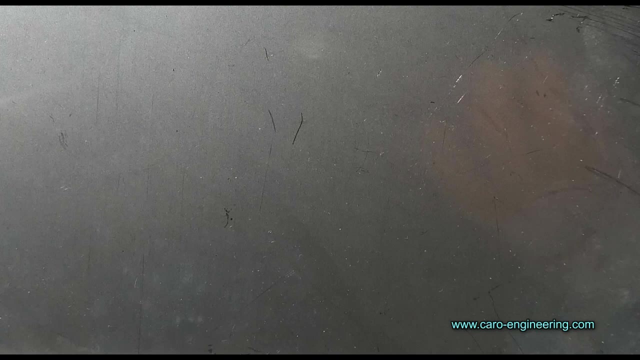 it back and forth, it will eventually break right where the notch is. So wherever possible, stress concentrations must be avoided. Surface roughness and scratches also cause stress concentrations. A smooth or polished surface is best. The material selection influences the fatigue life of a part as 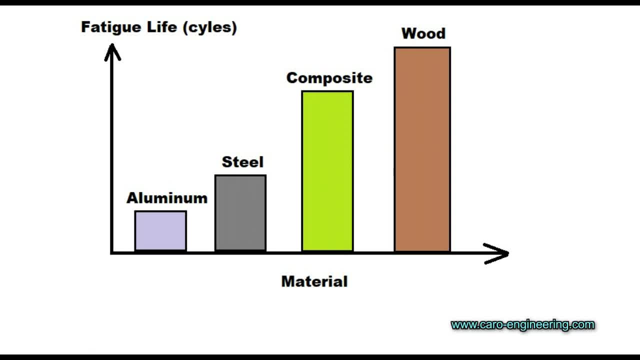 well. In general, aluminum is worse than steel. composite is better than metal. Wood comes out on top. After all, if trees fatigued, they would not get very old. If a part survives 10 million cycles, it can be considered safe for an infinite number of cycles. 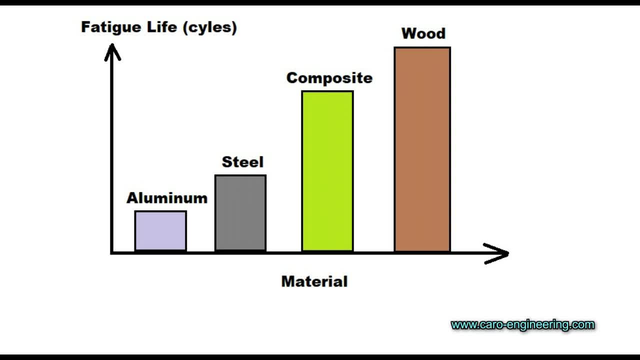 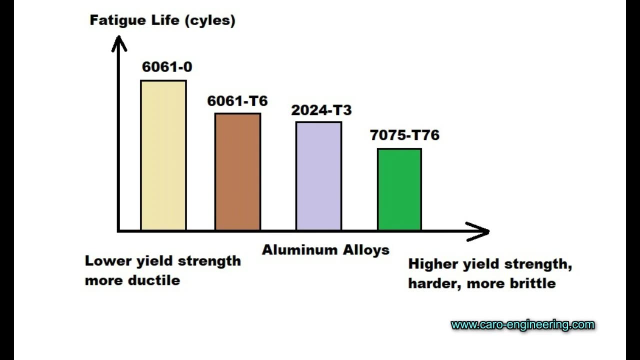 Materials that have high yield strength but are hard or brittle are worse than more ductile materials, even though they may have a lower yield strength. This is particularly important to remember when selecting aluminum alloys and tempers. These aluminum alloys are lined up with a thin layer of aluminum. The aluminum is 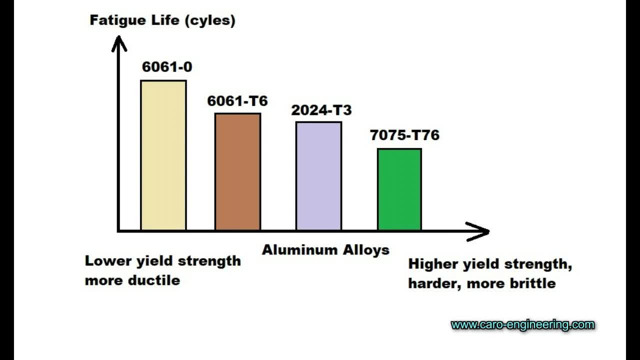 lined up in sequence from better to worse fatigue strength from left to right. Soft, easy to bend material with low yield strength is on the left, while alloys from the 7000 series, which have higher strength but are more brittle, are on the right side. 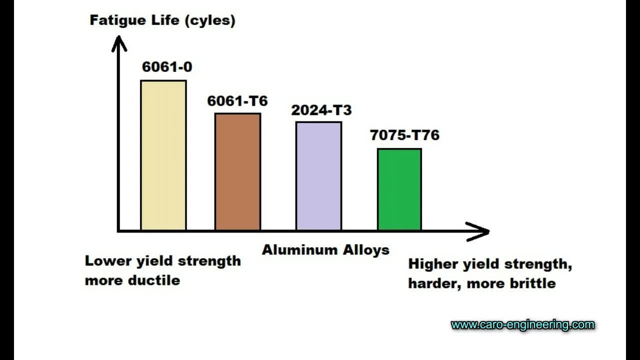 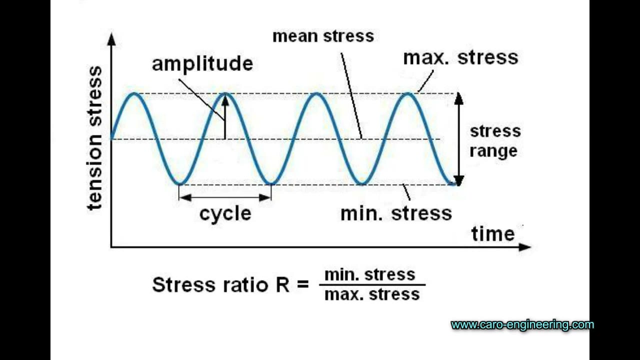 The 2024 alloy is a popular material used on airplanes because it offers the best compromise between strength and fatigue life. Aluminum parts in general do not achieve an infinite fatigue life and will eventually fail even from small stress amplitudes. The fatigue life of a material is determined through tests. Samples are subjected to load. 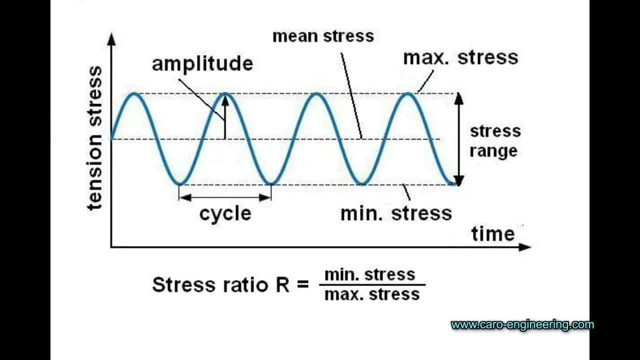 cycles of different magnitudes. In fatigue life analysis, it is important to distinguish the stress range, which is the difference between minimum and maximum stress, the stress amplitude and the maximum stress. It is the stress range, rather than the maximum stress, that drives fatigue damage. 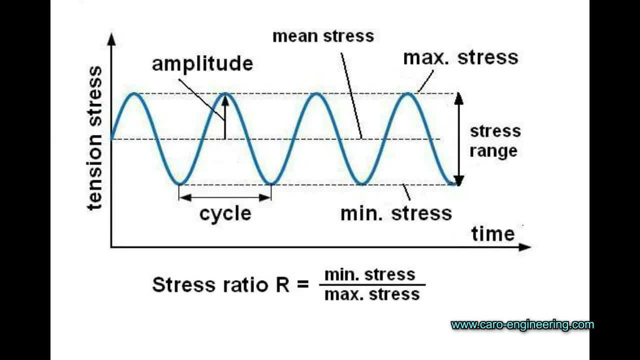 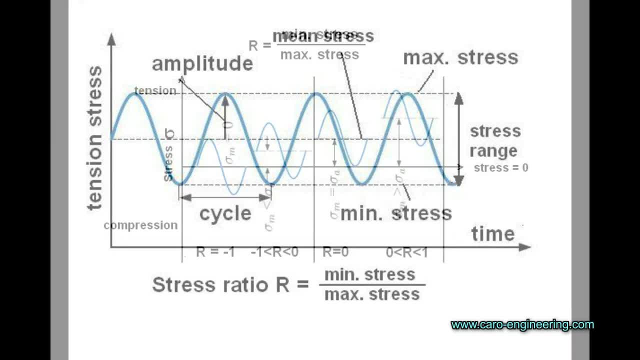 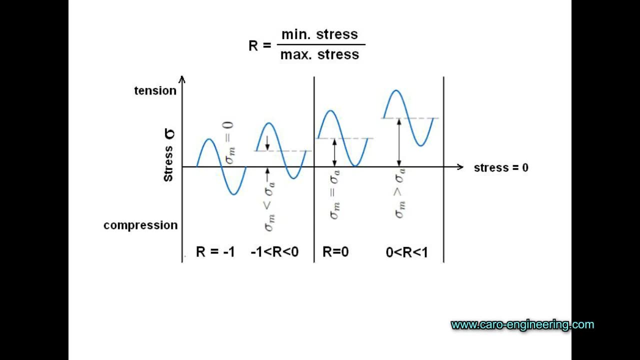 In flight. for the most part, turbulence provides the load cycles on an airplane and the stress range varies considerably for all of its parts. The stress ratio R, which is the minimum stress divided by the maximum stress, determines where the S-N curve will lie. Common stress ratios are between minus one and plus one. 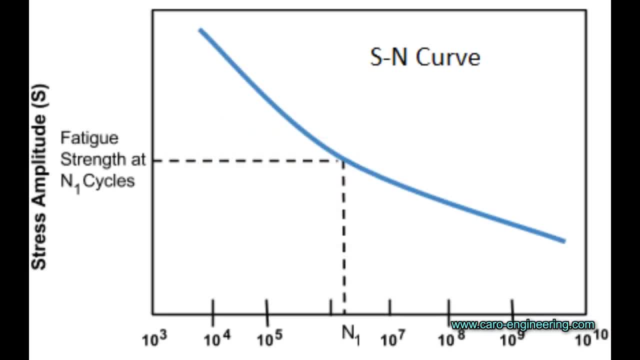 The fatigue characteristics of a material are shown in a chart called S-N curve. The X-axis shows the number of cycles at which a specimen will fail if it is tested with a stress range or amplitude shown on the Y-axis. The X-axis is usually shown in a log scale. This chart shows a comparison between aluminum. 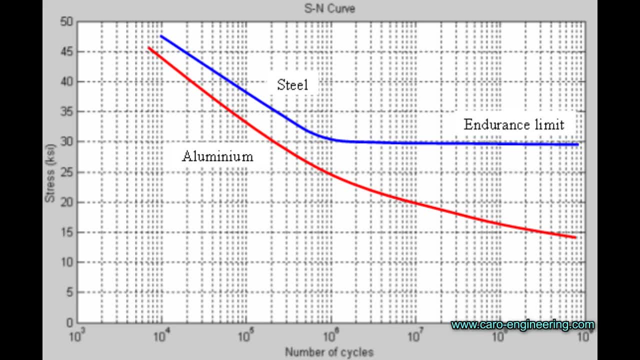 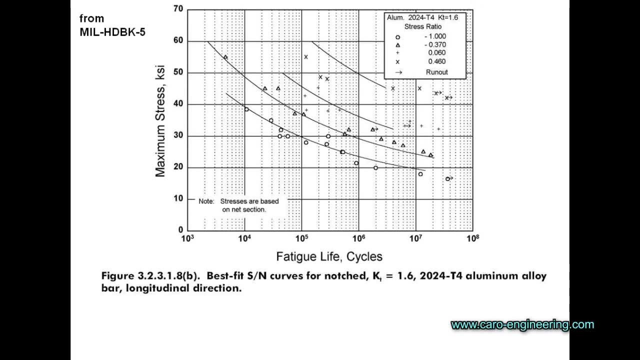 and steel. Steel may reach an endurance limit, while aluminum does not have this. The fatigue life curve for common structural aircraft materials can be found in mill handbook. 5. Metallic materials and elements for aerospace vehicle structures. It can be found online for free from various sources. 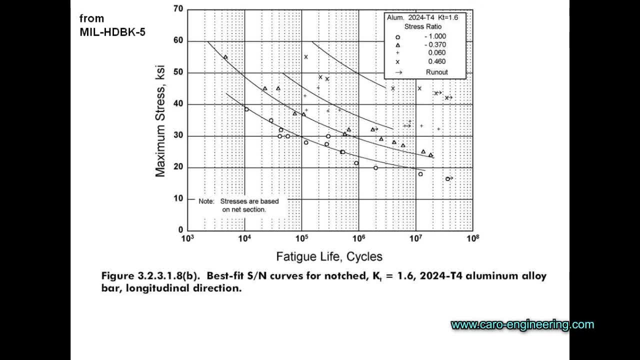 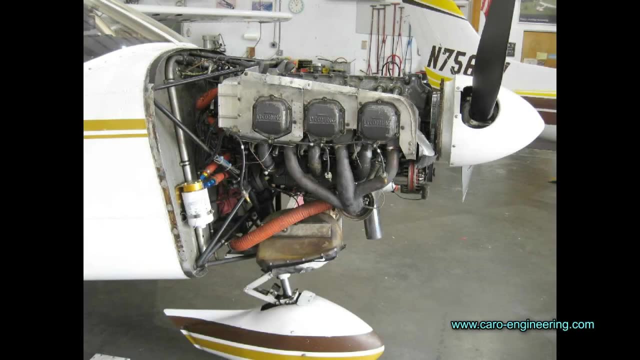 The example chart shown in the chart is for notched specimens for different stress ratios. Here the Y-axis shows maximum stress result of mechanical load cycles. Thermal load cycles can also cause fatigue damage in metals, for example in aircraft engines. Air-cooled engines go through large temperature changes. 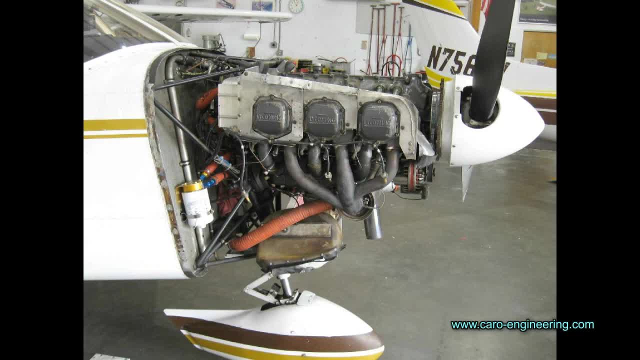 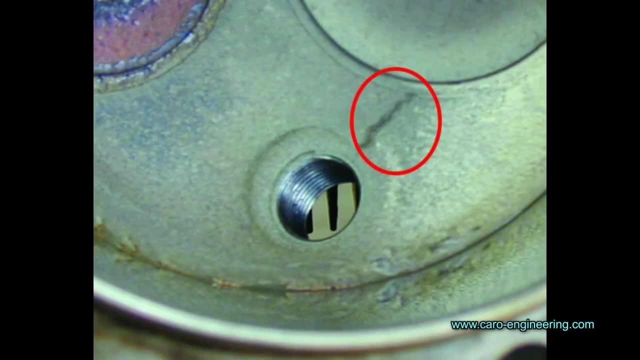 in addition to vibration, during which the material expands in contracts and fatigue, damage accumulates, The crankcase cylinders and cylinder heads and exhaust pipes are at risk. Once a crack shows up in a case, for example, it is an indication that it is near the end of its. 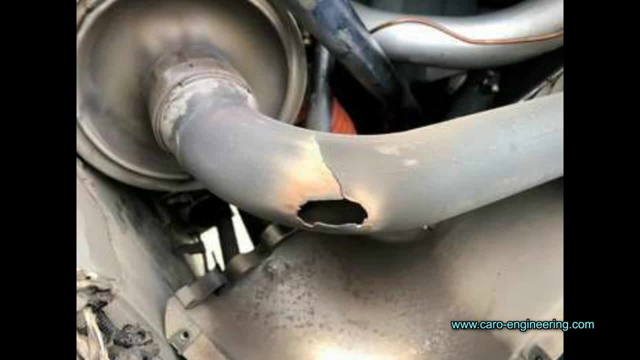 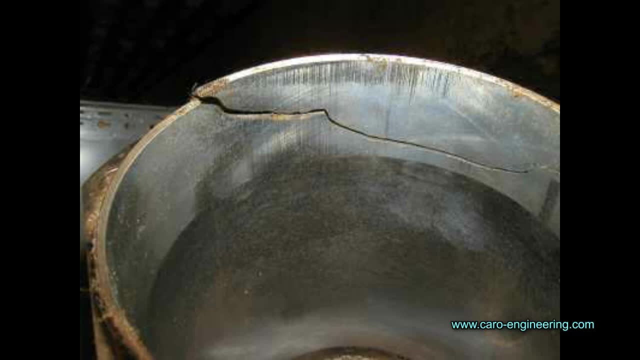 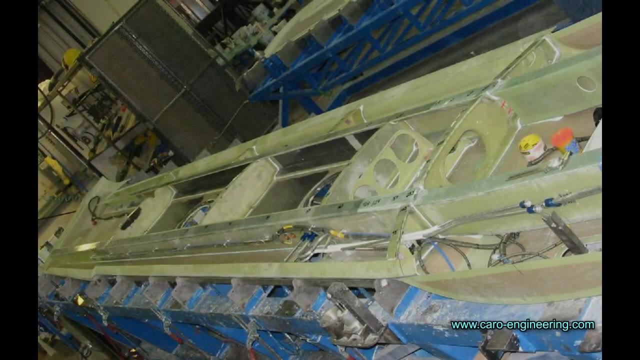 fatigue life. Even if the crack can be repaired, the rest of the material is probably not far behind and cracks may soon develop in other places. It is therefore best to replace the damaged part with a new one. Composite structures are more fatigue resistant because the load-bearing 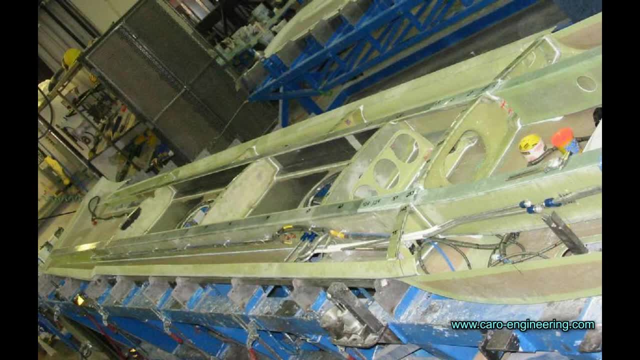 fibers are so small in diameter. Simply said, if one is damaged, there are many more to take over. The matrix, or resin, does fatigue, and here it is important to design the part to orient the fibers so that they are in the direction of the loads and the matrix only has the job of holding the fibers together. Additionally, 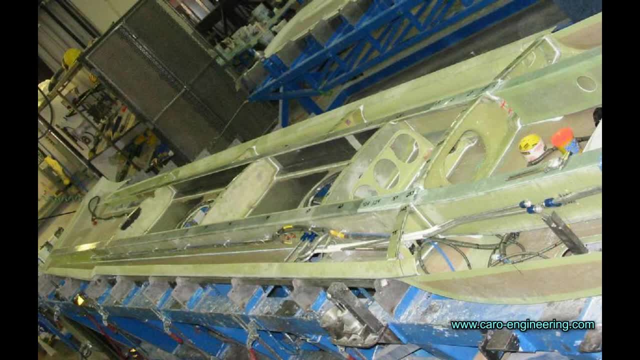 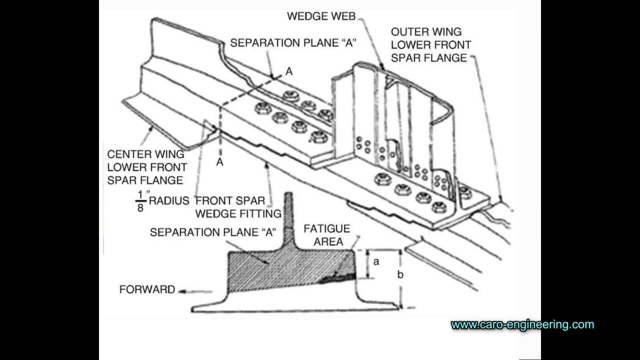 there are much fewer holes in composite structures, which equals fewer stress concentrations because the parts are bonded instead of riveted. The fatigue life of an airplane is typically set equal to the life of the highest stress part, the wing spar. The designer has to limit the maximum stress level in spar caps. 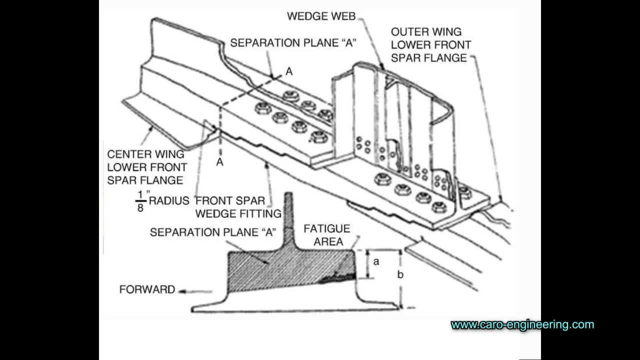 with considerations for stress concentrations to the desired number of cycles on the S-N curve for the material used. There is always a trade-off. If you select the high cycle number or more ductile material, the design maximum stress level is lower and the part has to be made thicker. 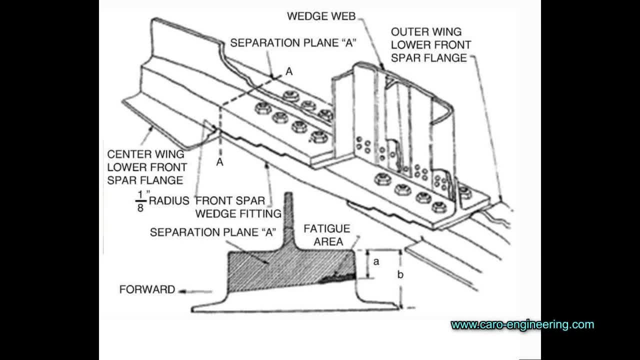 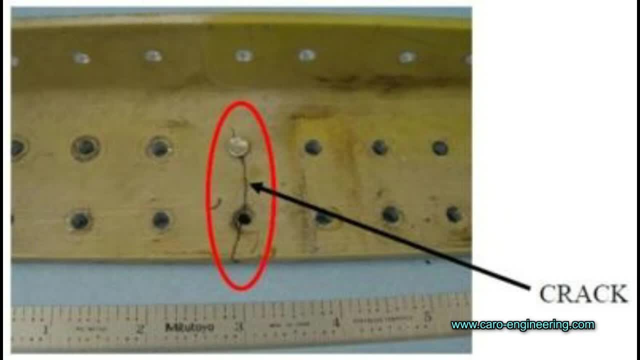 and heavier, or vice versa. For metal there is a fairly large difference between the load at failure of a new part and the load at failure of a fatigued part after many cycles. For wood and composite parts this difference is much lower. A good design fatigue life. for a small airplane is 10,000 hours. Obviously the fatigue life is much lower, but the design maximum stress level is lower. For metal, the design maximum stress level is lower and the part has to be made thicker. For metal, the design maximum stress level is lower and the part has to be made heavier. 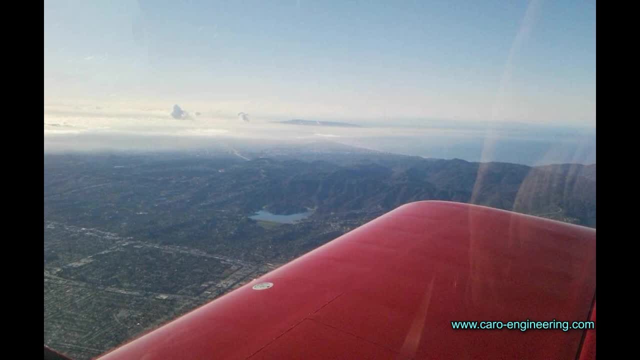 Obviously the designer cannot predict how many cycles the airplane will endure during its normal operation, so he will have to make some assumptions. A metal airplane that spends a lot of time in cruise in smooth air may not develop any cracks for 15,000 hours. Another airplane of the same model that spends all its life flying. 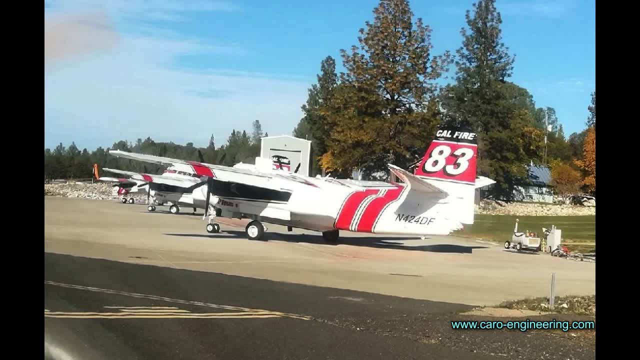 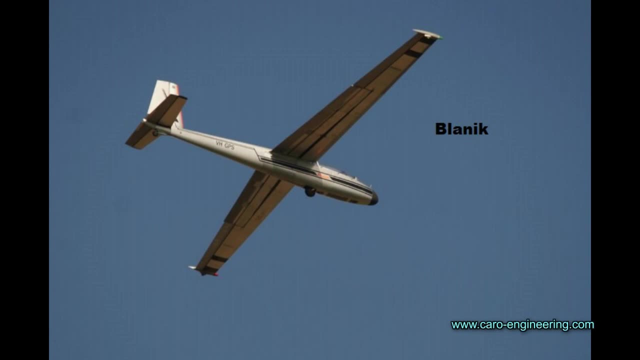 through turbulence or which is used for frequent aerobatics, may fail after a much lower number of flights, Because the airplane structure is much more complex than that of the samples which were used to determine the SN curves. there sometimes are surprises with high-time aircraft. This was the case for the all-aluminum Blahnik glider. 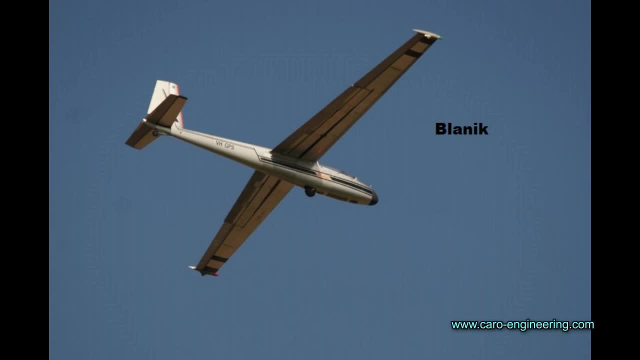 where a wing failed in flight from fatigue damage at the root. This resulted in limitations for the fleet: A maximum of 100 hours of aerobatics, a maximum of 25,000 winch launches and a maximum of 2,500 flight hours with two occupants. 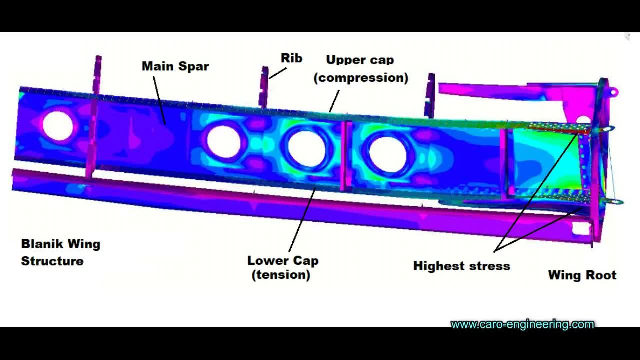 This picture shows stress analysis of the wing structure at limit load. The colors indicate where the highest stress is in the spar at the wing root. Critical for fatigue is only the lower spar cap, which is stressed in tension. A modification was developed to reinforce the critical area. 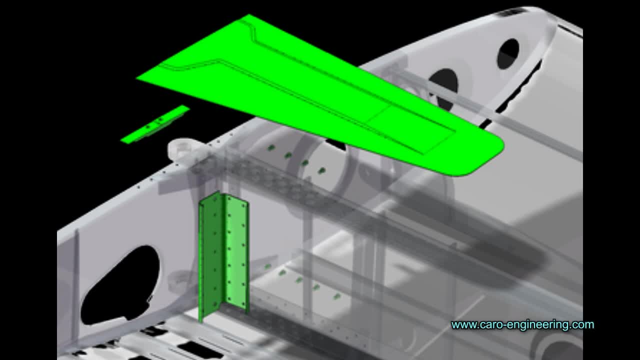 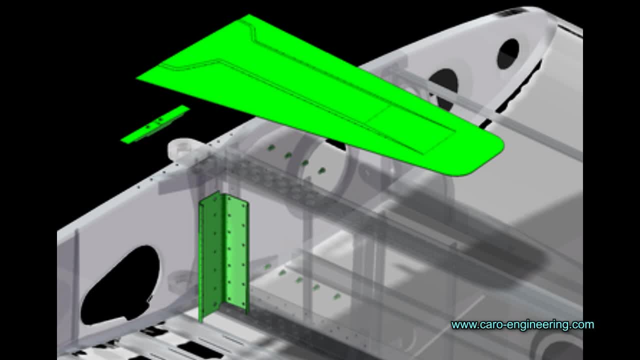 no aerobatics and life-extension to 5,000 hours useful life, or Some aerobatics and 3,750 hours of useful life. The modification consists of an additional root rip bracket, the addition and replacement of several highly loaded rivets. 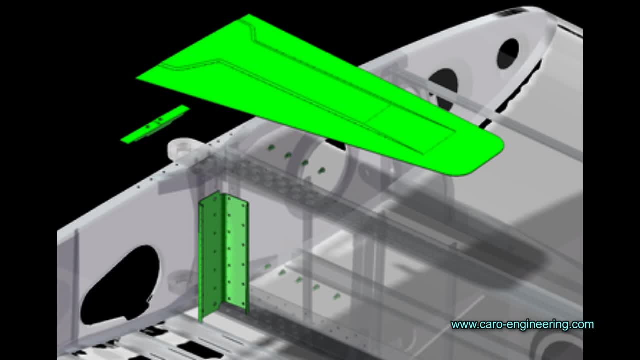 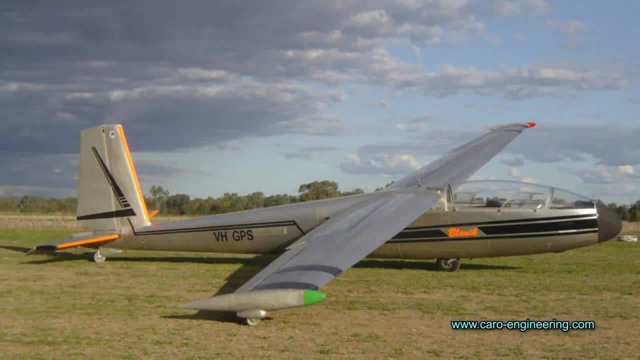 The modification consists of an additional root rip bracket, the addition and replacement of several highly loaded rivets- climbing equipment part flなんです- and additional kyslt 미러� eliminations nowadays and an additional reinforcement plate attached to the lower spar cap at the wing root. 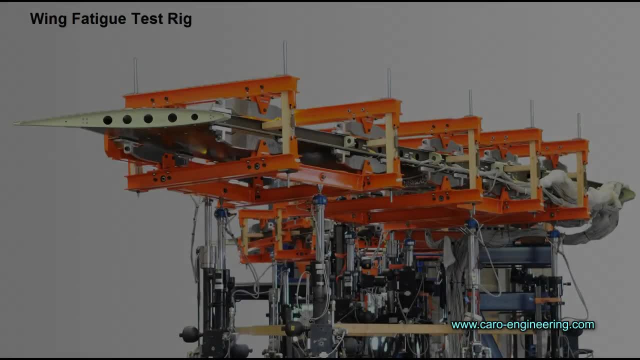 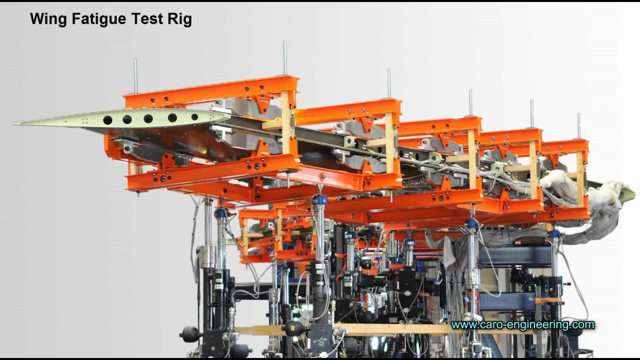 The fatigue life of a new airplane is estimated by analysis and simulated by testing components like complete wings or fuselages, with a cyclic load spectrum to failure. If, for example, a wing fails on the test stand after 18,000 simulated hours at various load cycles. 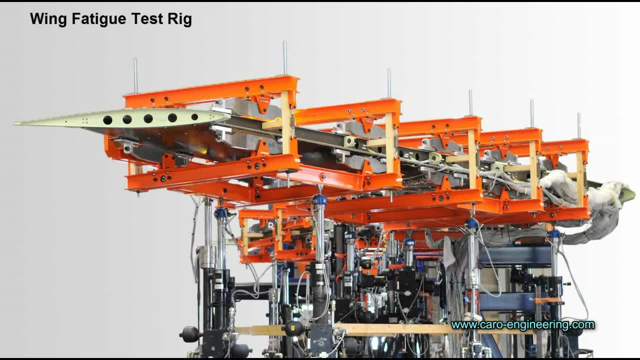 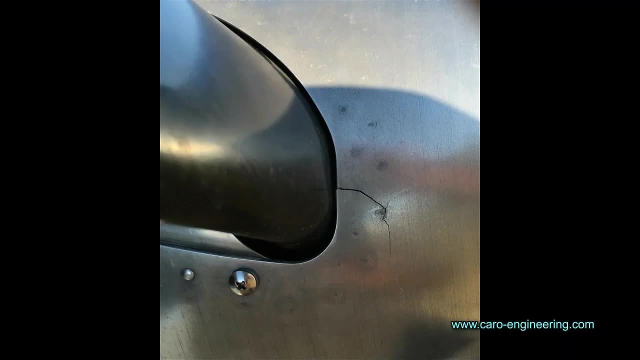 its service fatigue life is this number divided by a safety factor, typically 3,, so it can safely fly for 6,000 hours. Even before the design fatigue life is reached. parts of an airplane can develop visible cracks. Common places for cracks to show up are aluminum spinners and baffling because of the high vibration level in the engine compartment. 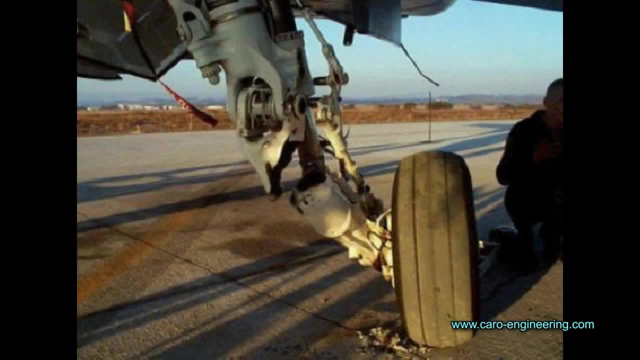 Once a crack is found, the part should be repaired. If you find a crack in one part of an airplane, you have to assume that the airplane has already accumulated a certain amount of fatigue damage. It should be thoroughly inspected in critical areas such as lower wing spar caps and connections for visible cracks. 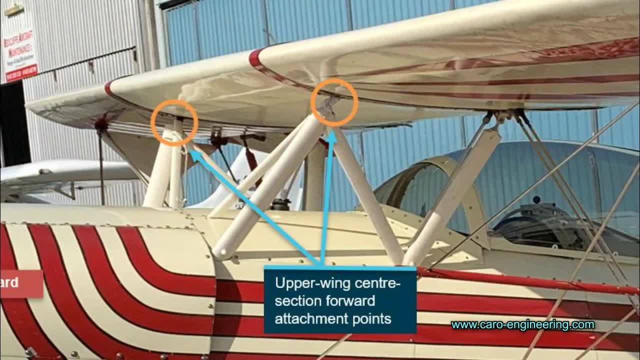 Another example of fatigue damage was found on the upper wing connection of a biplane where the bolts failed. If possible, evaluate the risk of a catastrophic failure based on the airplane's operational history- like many low-level flights and turbulence, aerobatics or primary flight training, and the service record of other airplanes of the same model. 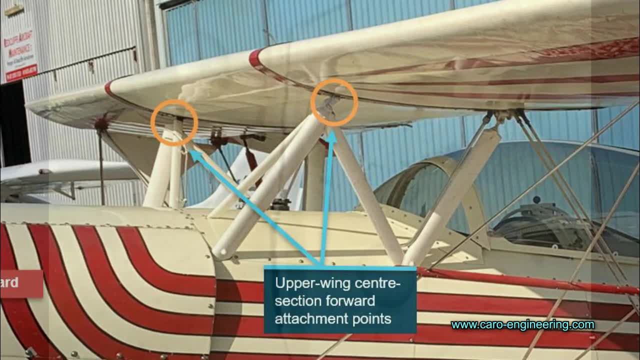 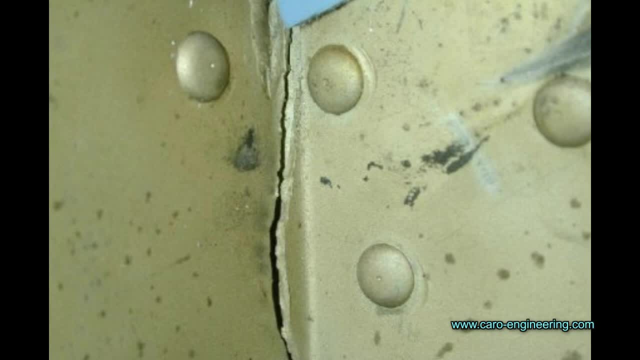 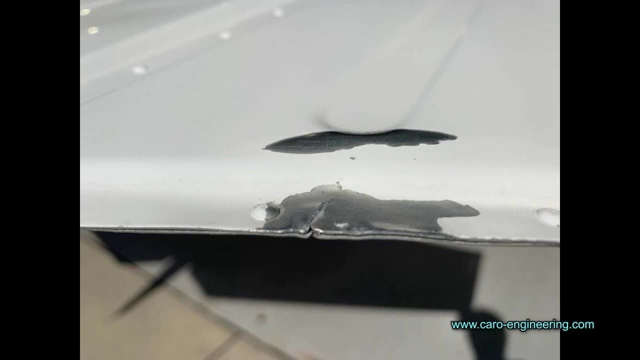 Other areas that are at risk are thin-walled aluminum ribs and control surfaces, especially in those areas that are subjected to additional loads from engine vibrations, prop wash or flexing. A part that is weakened by corrosion will develop cracks and fail much sooner than an uncorroded part. 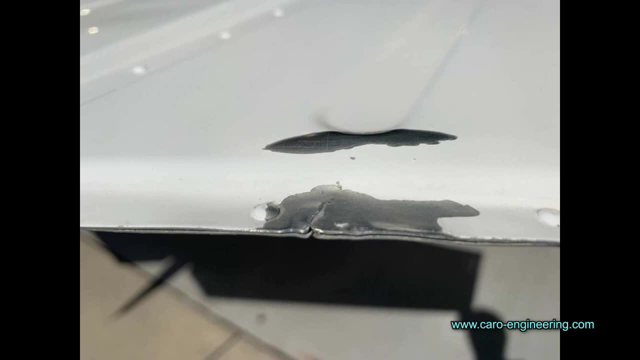 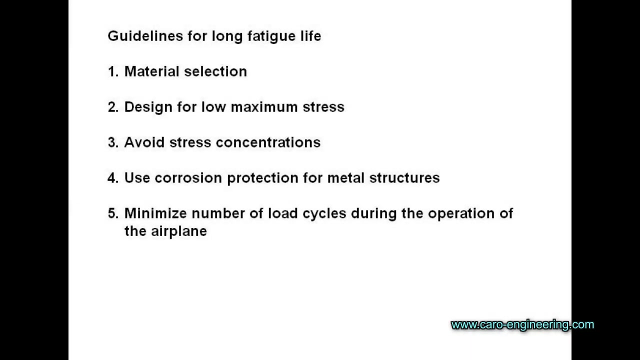 Here it helps to inspect the structure of a metal airplane frequently and use corrosion protection where possible. Once there is fatigue damage, it cannot be removed. Here is a summary of guidelines for good fatigue life of an airplane: Material selection. Design for low maximum stress.